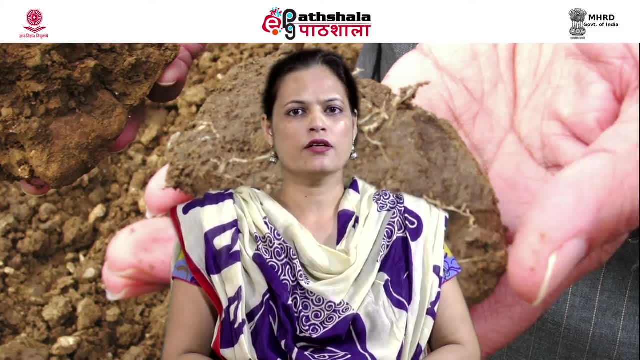 and physical withering, transported and located, is termed as transformed soil. The formation of soil. it can also be seen as the product of withering. Then, after withering, the structural formation of soil takes place. After the formation of the structure of soil, it will undergo the 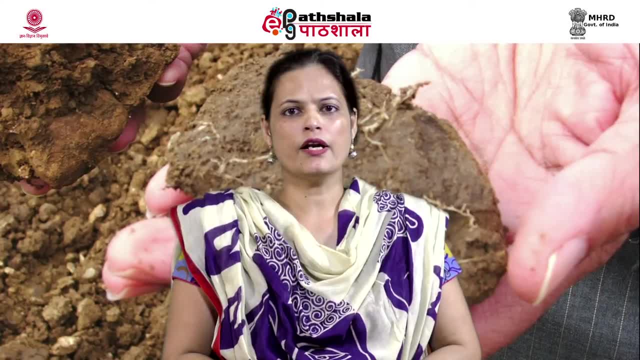 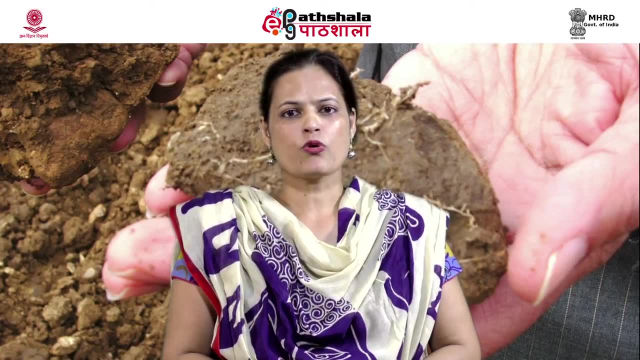 process of formation of horizons or layering, Then the movement and translocation of soil takes place In the soil. physical and chemical withering, climatic conditions also plays very important role. On the other hand, water it is also. it also plays important role by showing. 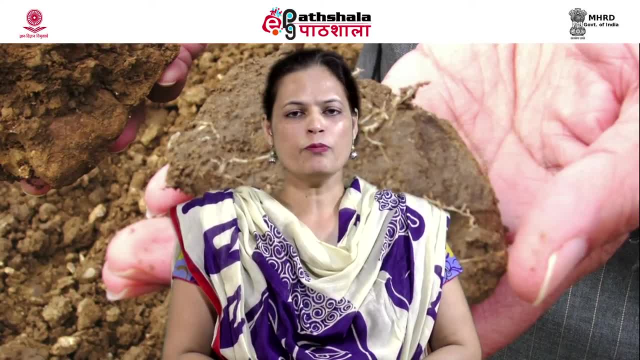 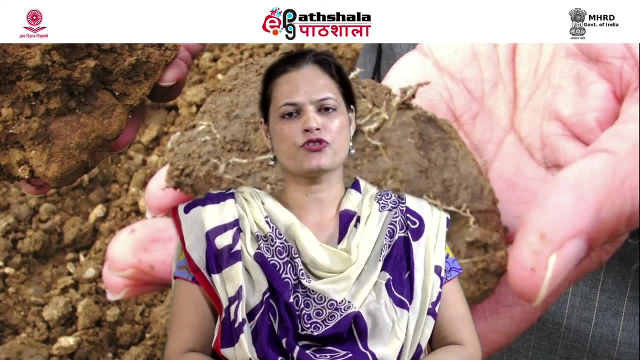 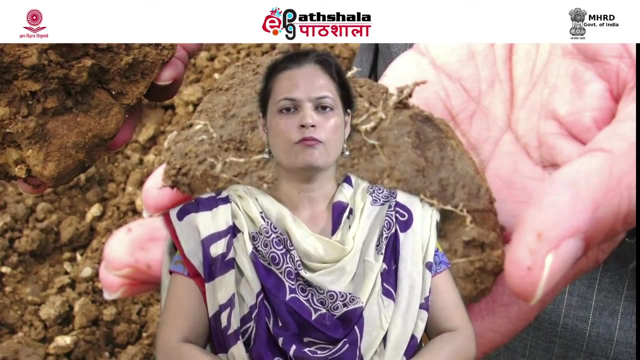 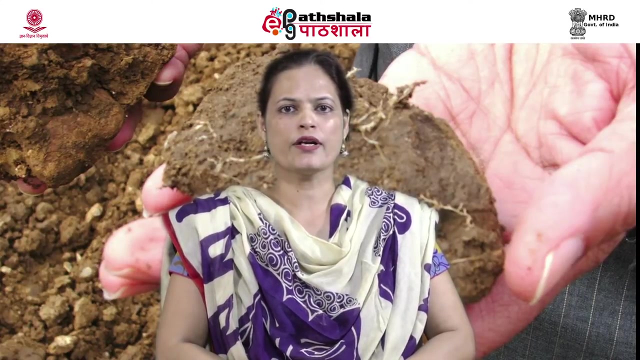 its involvement in soil development through dissolution, precipitation, erosion, transportation and deposition. The soil is also having three phases: Solid, liquid and gaseous phase. Moreover, the soil scientist they prefer to include five important components while studying the soil formation, And these components are: 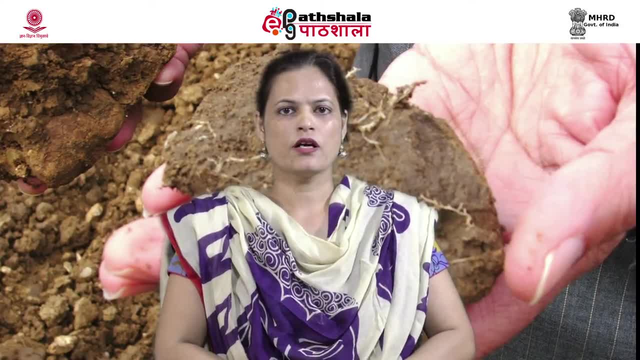 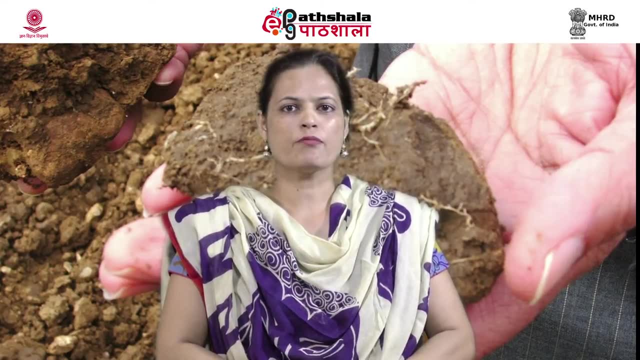 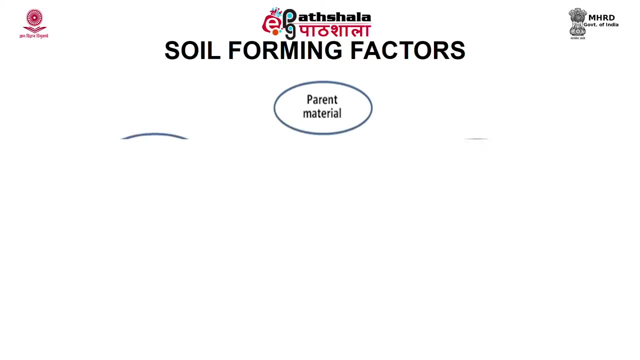 parent material organisms, time, climate and relief. On the other hand, soil also contains five important components which are very important for the healthy soil. Now we take the process of soil formation. Soil formation develops as a result of interplay of five factors, which I have already told. 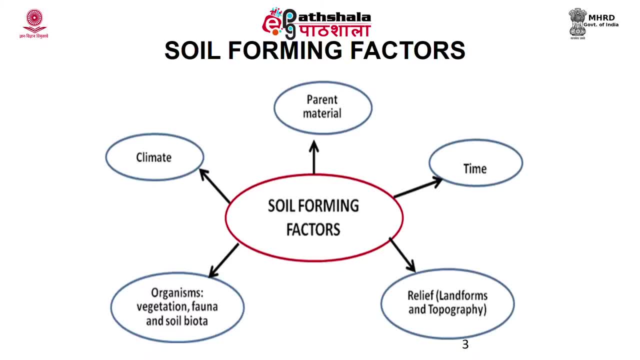 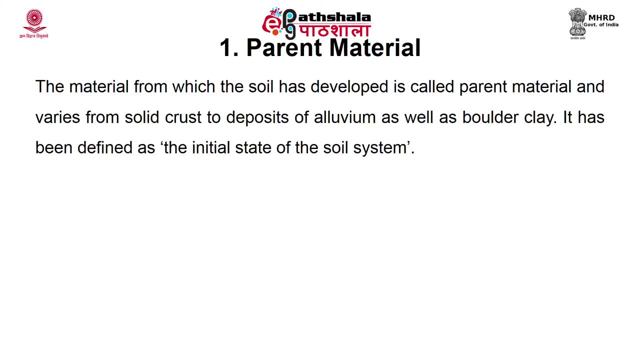 as parent material, climate, organism relief and time. Now, first we will take the parent material. This is the material from which the soil has developed and can vary from solid rocks to deposits. It has been defined as the initial state of soil system. 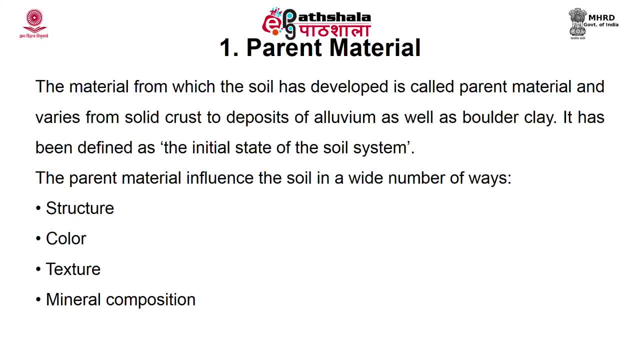 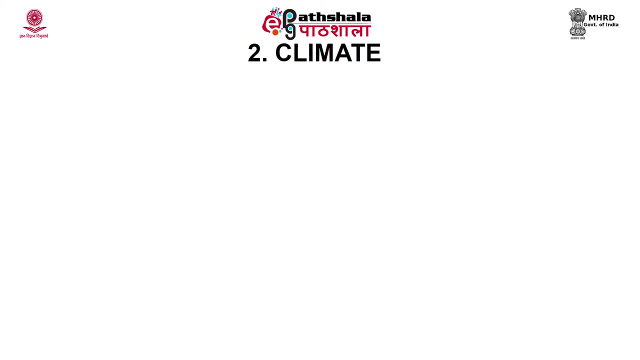 The parent material can influence the soil in number of ways, For example, color, texture, structure, mineral composition, permeability, soil structure, aging output. This soil has developed an old red sandstone and so has derived its distinguished color from its parent material, as shown in the figure. 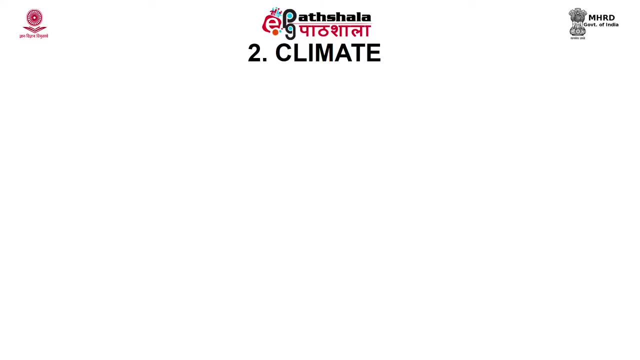 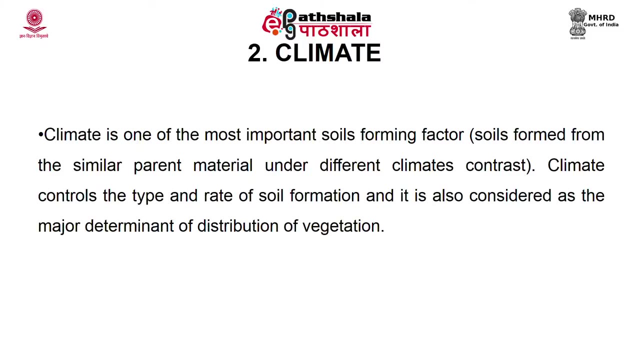 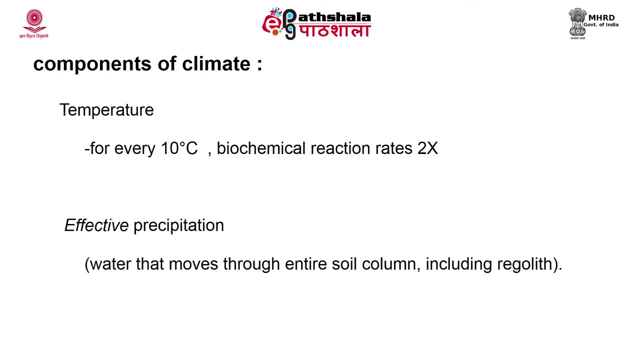 Climate – this is probably the most important factor. Climate governs the rate and type of soil formation and is also the main determinant of vegetation distribution. On the other hand, temperature determines the rate of reaction, Chemical and Balanced decay, and so has influence on withering and humification of the soil. third, that 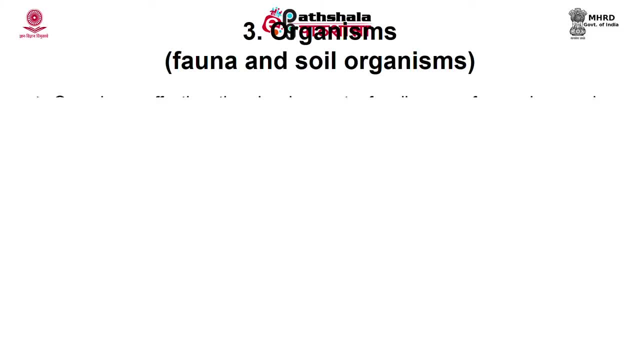 is our organisms which play important role in soil formation. organisms influence soil development. range from microscopic bacteria to large animals, including man. microorganisms such as bacteria and fungi assist in the decomposition of plant litter. this litter is mixed into the soil by my microorganisms, such as our worms and beetles, say. soil origins are less. 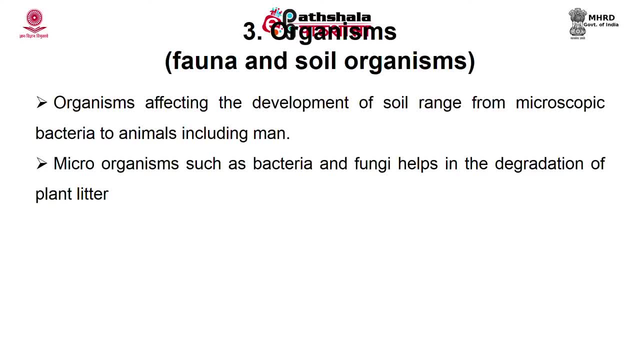 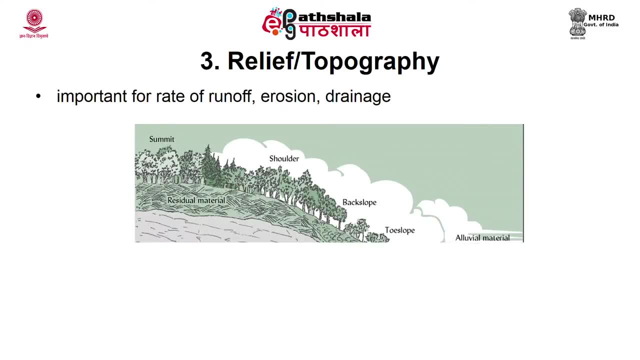 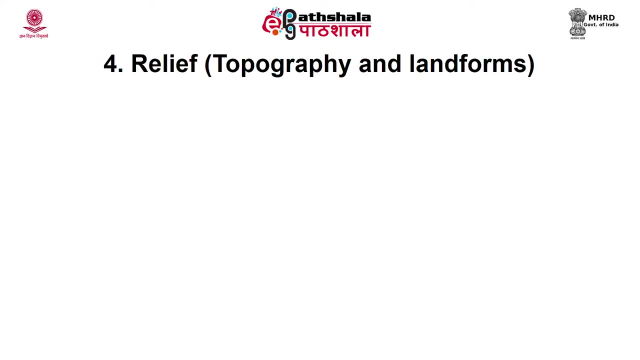 distinct when there is much soil organism activity. another important point is relief, that is, landforms and topography of a particular area. relief is not statistic. it is a dynamic system. it influence soil profile thickness. it has an effect on climate, which is also a soil forming factor. 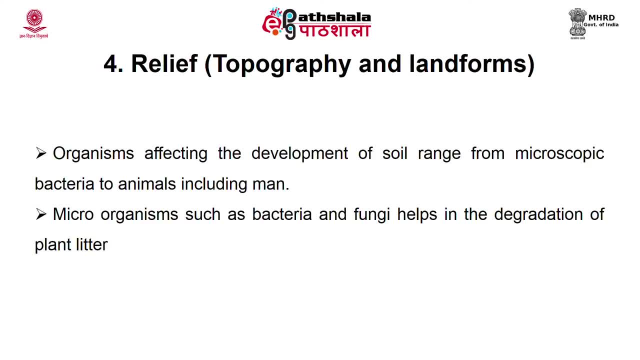 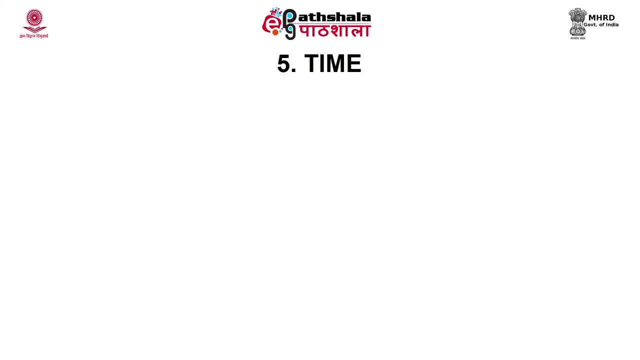 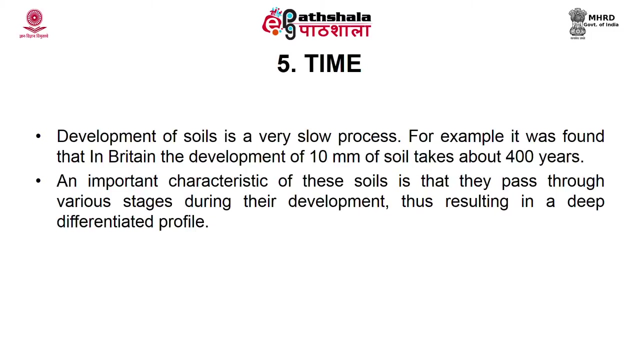 gradient. The gradient affects runoff, percolation and mass movement. It influence aspect which creates microclimatic conditions of the area. Another important point factor is time. Soil develops very slowly. For example, if we take the example of Britain, it takes about 400 years for 10 mm of soil. 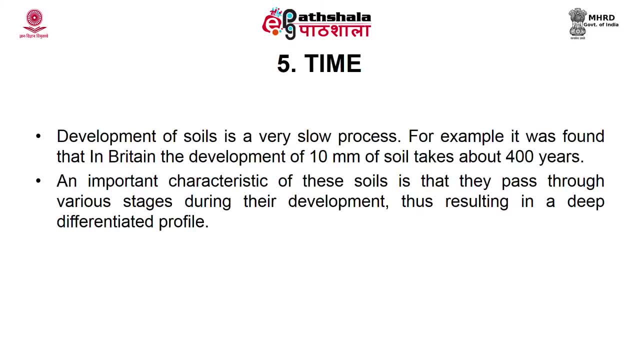 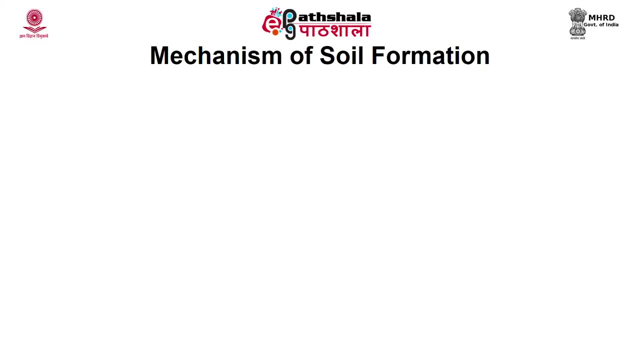 to develop. Young soil retains many of the characteristics of the parent material. An important feature of soil is that they passes through a number of stages as they develop, resulting in a deep profile with many well differentiated. Now we come to the next process, that is, mechanism of soil formation. 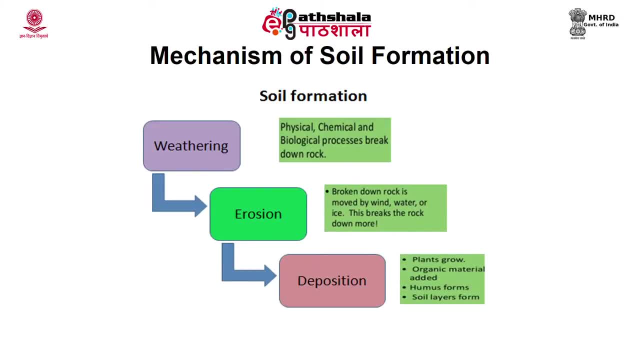 Soil develop through a series of changes. All soil originates from a parent material, which is a deposit at the surface of earth. Parent material can be withered, bed rocks or small materials brought by strong winds, flowing rivers or moving glaciers. The simple compound relieved by withering becomes food source for soil organisms such 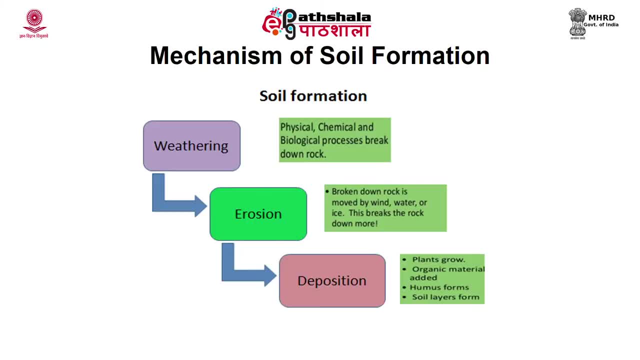 as bacteria and fungi. The remains of the dead organisms accumulate in the parent material and turns into an organic matter or humus, TOMOS. 0.00PERCENT Soil Formation through Withering in 말�ing erosion or deposition processes. now, first we'll take the withering. withering is the breakdown and 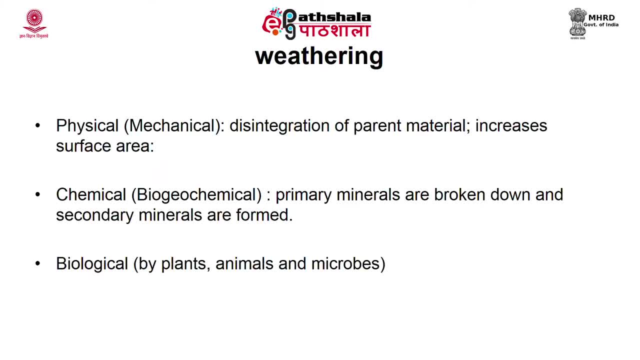 alteration of rocks and minerals at the near of the earth surface into products that are more in equilibrium with the condition found in this environment. withering is the first step for a number of geomorphic and biogeochemical processes. the product of withering are a major source of. 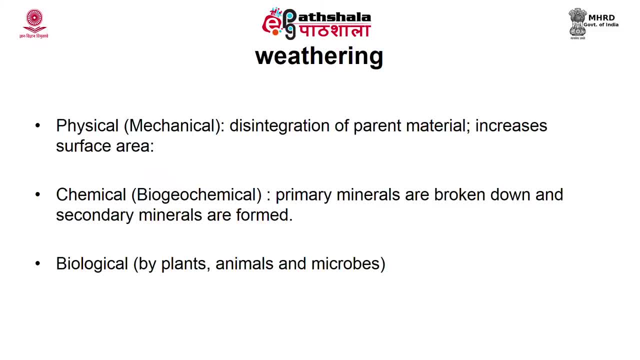 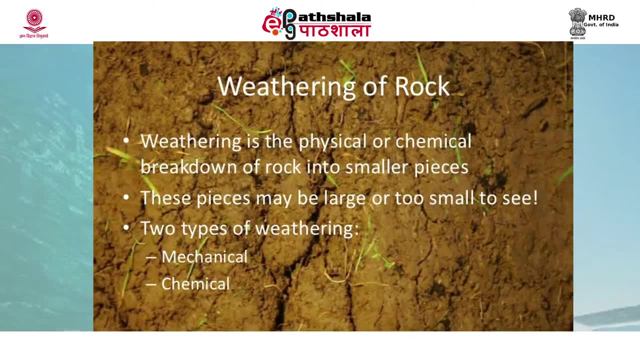 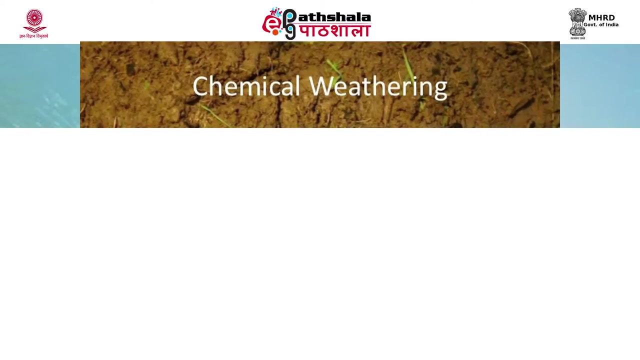 sediments for erosion and deposition. withering also contributes to formation of soil by providing mineral particles like sand, selt and clay. there are three broad categories of mechanism of withering. that is, physical, chemical and biological. now we'll take all these mechanisms one by one. first we'll take chemical withering. chemical withering involves the alteration 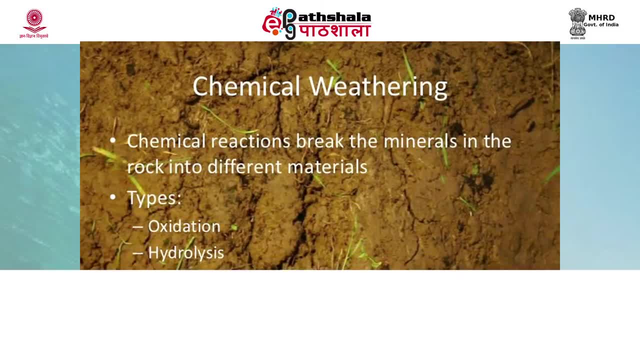 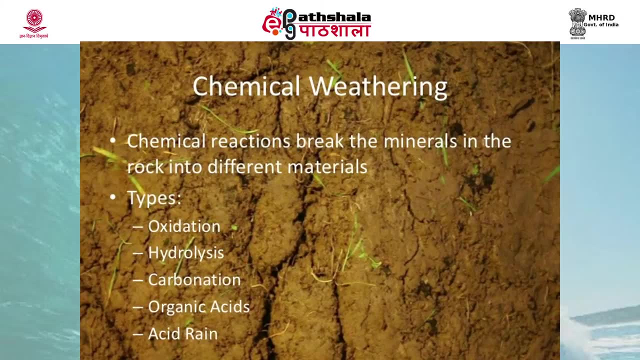 of the chemicals and mineralogy composition of withered material. A number of different process can results in chemical withering. The common chemical withering processes are hydrolysis, oxidation, reduction, hydration, carbonation and solution. Now we will take one by one these processes. Hydrolysis is 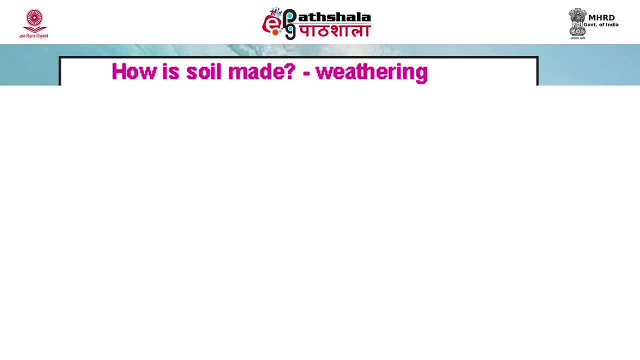 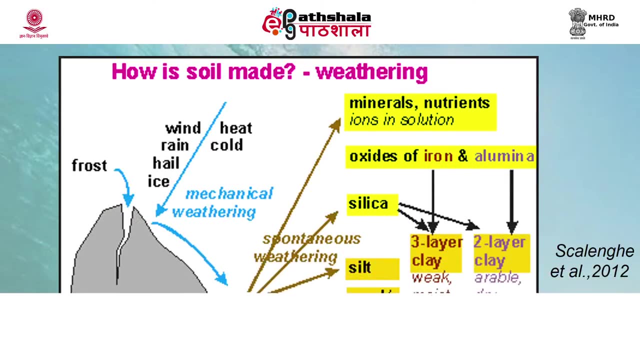 the withering of withering reaction that occurs when the two surface of water compound meets. It involves the reaction between mineral ions and the ions of water and results in the decomposition of the rock surface by forming new compounds. Hydrolysis is specially effective in the withering. 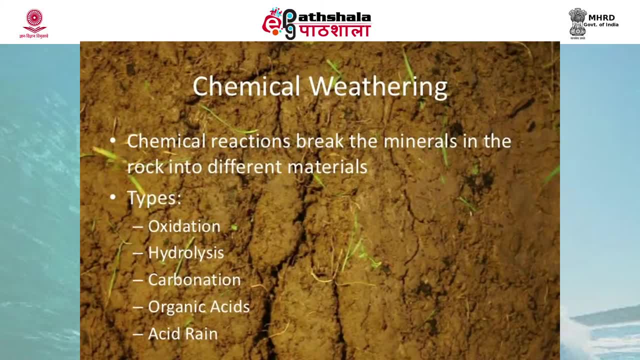 of common silicates and ammonia- silicate minerals because of their electrically charged crystal surfaces. Oxidation is the reaction that occurs between the compound and oxygen. The net result of this reaction is the removal of one or more oxygens from the surface of the rock. 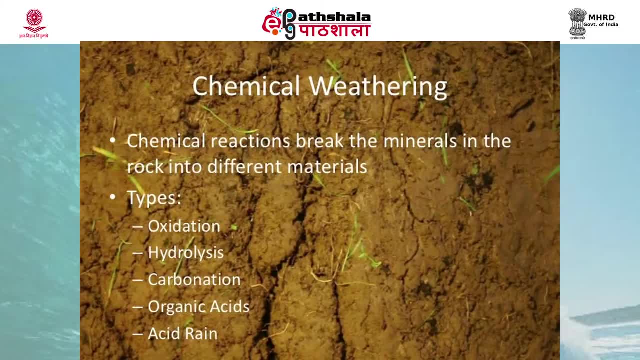 Now let us see what are the common oxygens in hydrolysis. Hydrolysis are oxygens that are exposed to four electrons from a compound, which causes the structure to be less rigid and increasingly unstable. The most common oxides are those of iron and aluminium giving 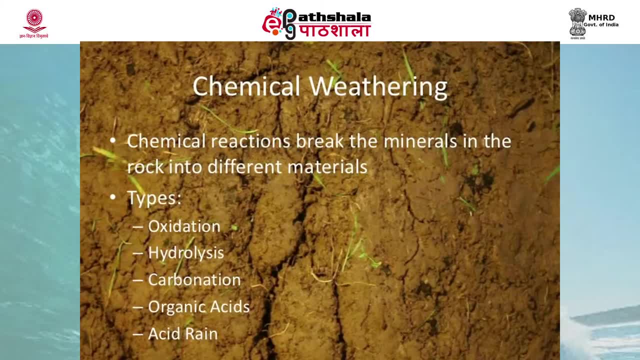 red and yellow staining to the soil and is quite common in tropical regions which have high temperature and precipitation. Hydrolysis is a process of withering of a material with within an oxygen cell by receiving a moistened cream for the final麹 Bombs. When this process is carried out, the vomits. 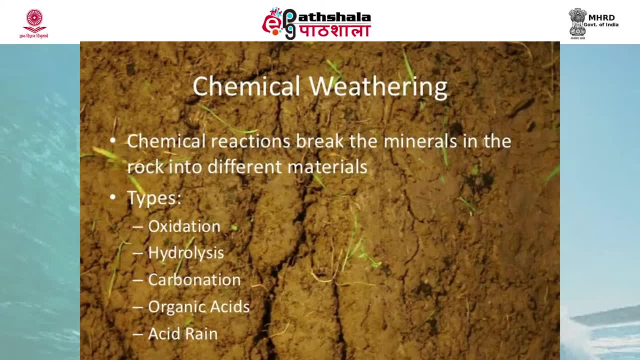 are realized by those oxygens which are used for the production of the material. Now we will take Hydration. Hydration involves the rigid attachment of Hydrogen and Hydronium ions. In many situations, the hydrogen and hydroxide ions become a structural part of the crystal. 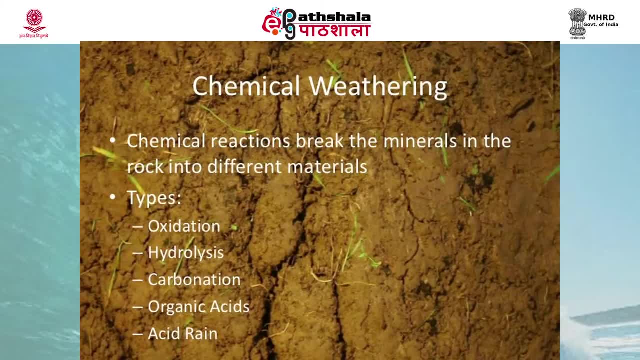 lattice of the mineral. Next, carbonation is the reaction of carbonate and bicarbonate ions with minerals. The formation of carbonate usually takes place as a result of other chemical processes. Carbonation is especially active when the reaction environment is abundant with carbon dioxide. Another important process that is now physical withering. 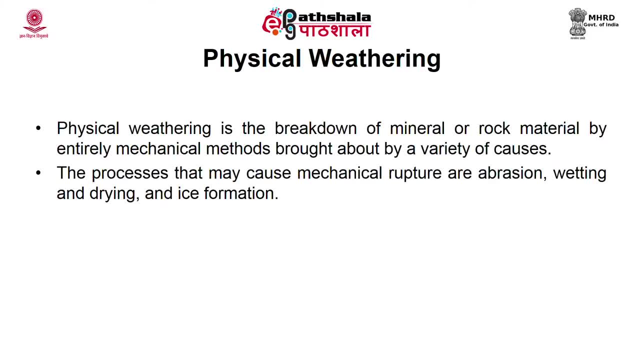 Physical withering is the breakdown of minerals or rock material by entirely mechanical methods, brought about by a variety of causes. Some of the forces originate within the rock or minerals, while others are applied externally. Both of these stress lead a strain and the rupture of the rock. 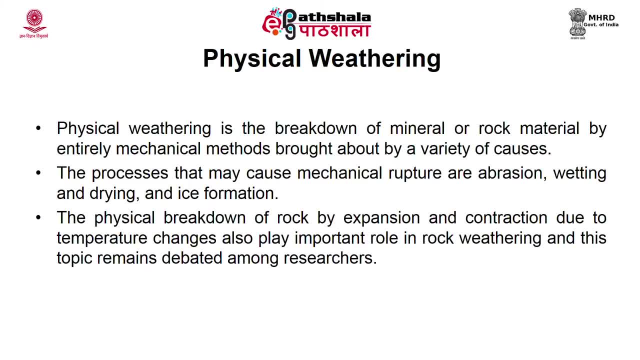 The process that may cause mechanical damage, Chemical rupture or abrasion, wetting and drying and ice formation. The physical breakdown of rock by their expansion and contraction due to the diurnal temperature changes is one of the most keenly debated topic in the rock weeding research also known. 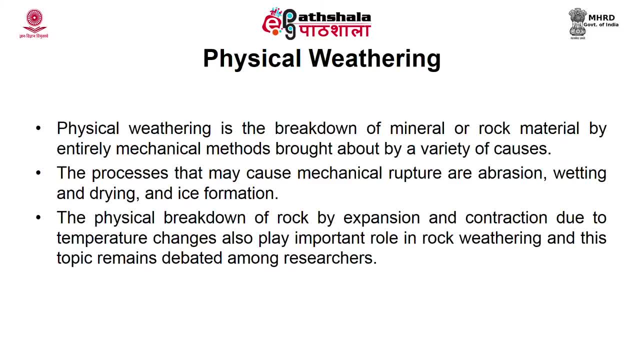 as insulation weathering. It is the result of the physical inability of rock to conduct heat well. This inability to conduct heat well is the result of the physical inability of rock to conduct heat well. The ability to conduct heat results in differential rates of expansion and contraction. 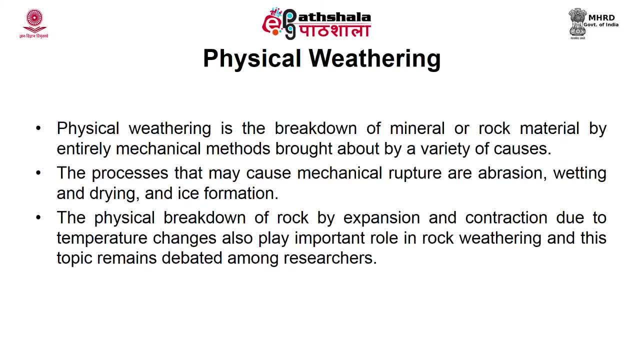 Thus, the surface of the rock expands more than its interior, and this stress will eventually cause rock to rupture. Alternate wetting and drying of rock, sometimes known as slacking, can be a very important factor in withering. Slacking occurs by the mechanism of ordered water, which is the accumulation of such water. 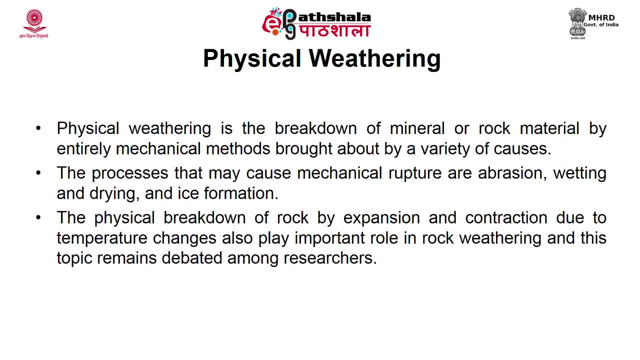 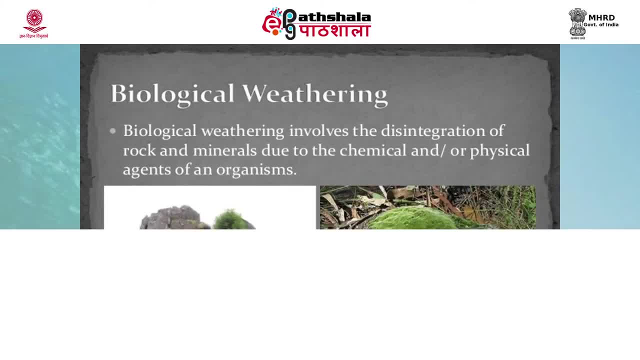 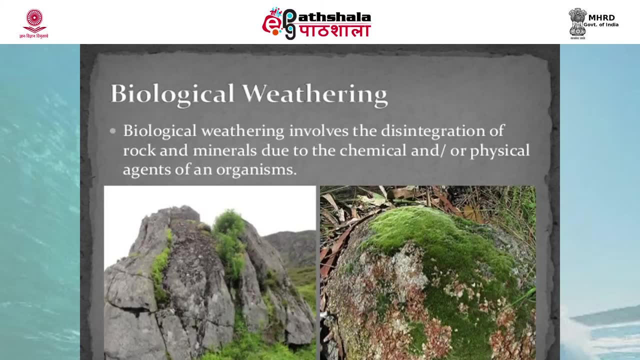 successive layers of water molecules in between the mineral grains of the rock. Another process, that is our biological withering. Biological withering involves the disintegration of rocks and minerals due to the chemical or physical agents of an organism. The types of organisms that can cause withering range from bacteria to plant to soil plants. 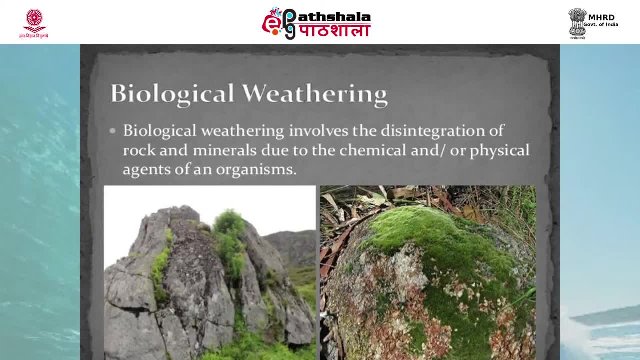 to animals. Biological processes, root penetration and animal burrowing are some of the processes which are determinants to this biological withering process. The organic compounds having acidifying molecules that corrode rock minerals and, as such, makes them weak and prone to disintegration, are also the main types of biological withering. 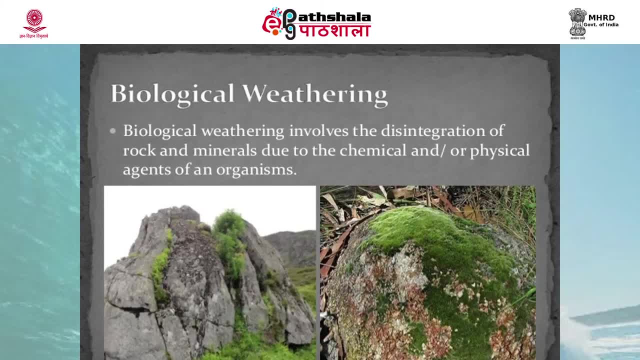 Some of the main types of biological withering processes are growing plant roots. It is common to see some roots growing within the face of a rock Well. such plant activity contributes to biological withering. The roots of plants and trees penetrate into the soil in search of nutrient and water. 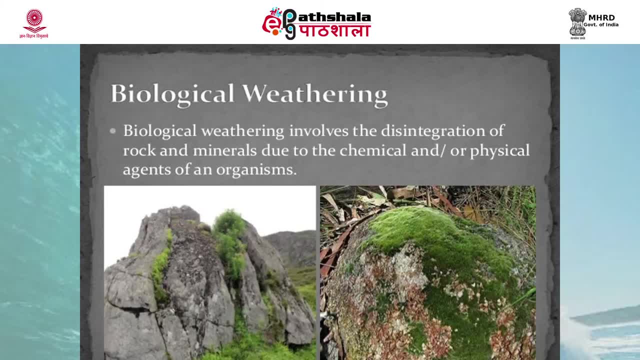 As the root penetrates the soil they go through cracks or joints in the rocks and as they grow they progressively crack the rock apart. Bigger growing roots can also exert pressure on the adjacent roots- See description of the video for more details. rocks- Some plant roots also emit organic acids that aid to dissolve the rock material. 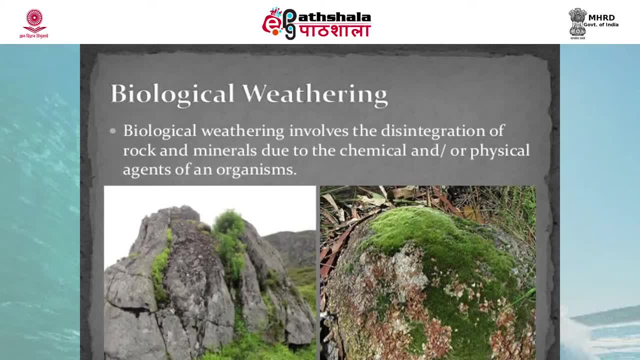 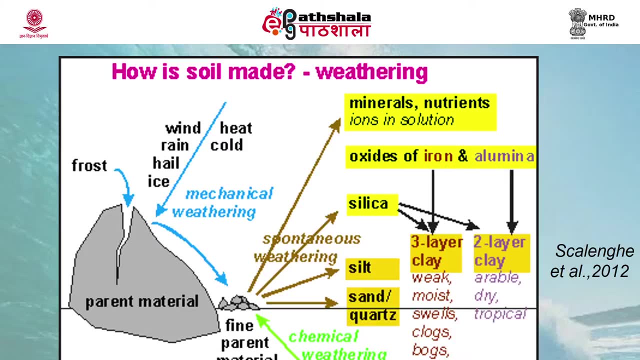 Another factor: microbial activity. Some plant microbial activity release organic acidic compounds. These compounds can break down iron and aluminium minerals in the rocks. Microscopic organisms like algae, moss, lichens and bacteria are such kind of plant. They grow on the surface. 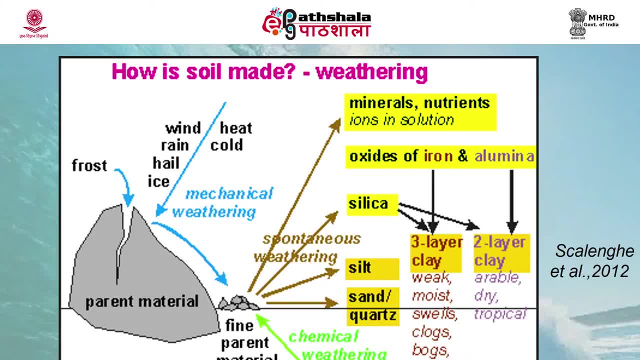 of the rocks and produce organic chemicals that are capable of breaking down the outer layer of the rocks by altering the rocks chemical composition, The process of biological withering, since it is a biological in nature. beside these microscopic organisms are bring about moist chemical microenvironment which engrace the chemical and the soil. 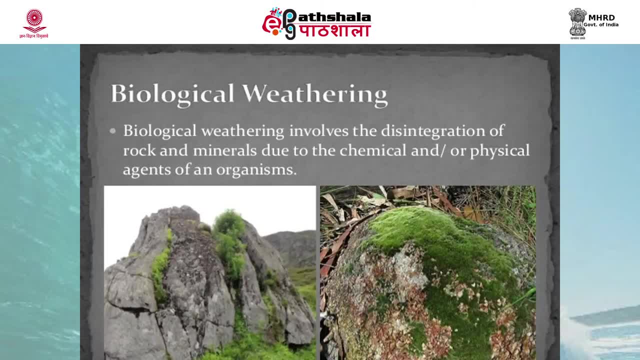 And physical breakdown of the rock surfaces. Burrowing animals are also plays important role in biological withering, such as moles, squirrels and rabbits can speed up the development of fissures. Many animals, such as Pidog shells, drills into the rocks for protection either. 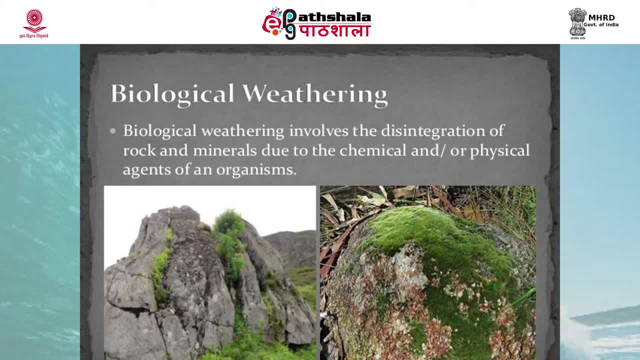 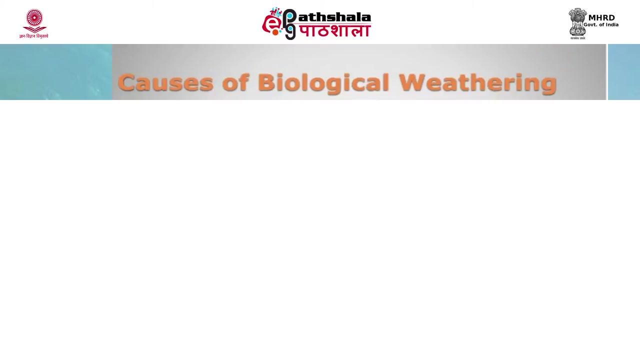 by releasing acid to dissolve the rocks or fragmenting away the rock grains. These animals activities can create fissures in the rocks and also eat away the rock. As this process continues, gaps and holes develop within the rocks, further exposing the rocks to chemical, biological and physical withering. Human activities are also considered to be. 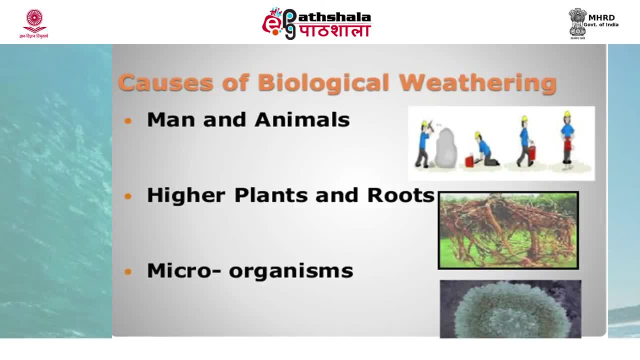 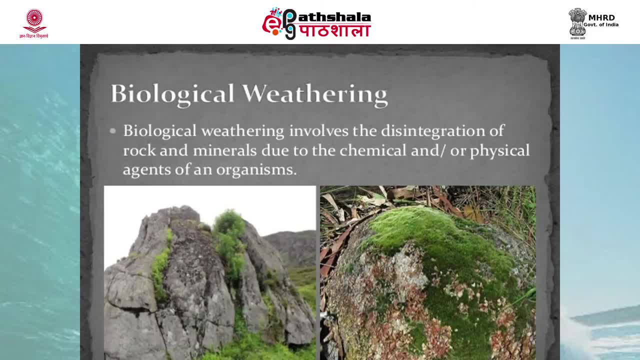 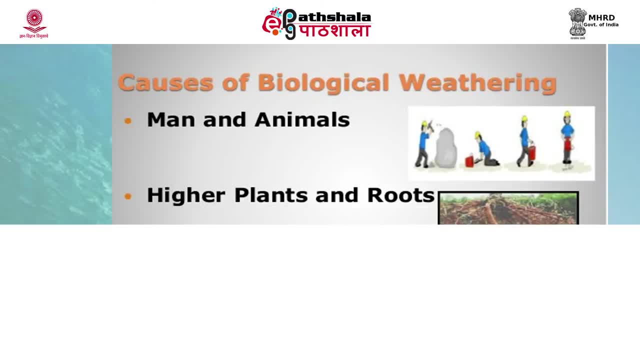 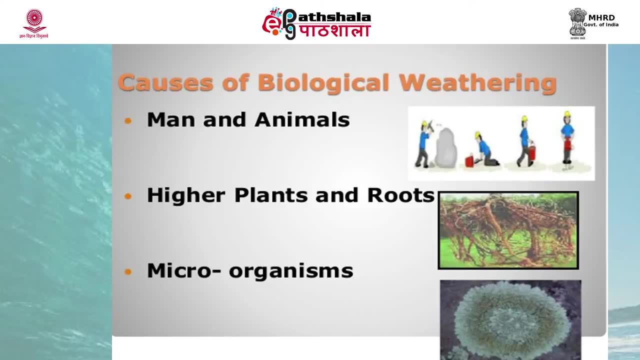 materials by the consumption of soil particles by animals. Particles can also fracture because of animals burrowing or by the pressure put forth by growing roots. Second point: movement and mixing of materials. Many large soil organisms cause the movement of soil particles. This movement can introduce the material to different withering processes found at distinct 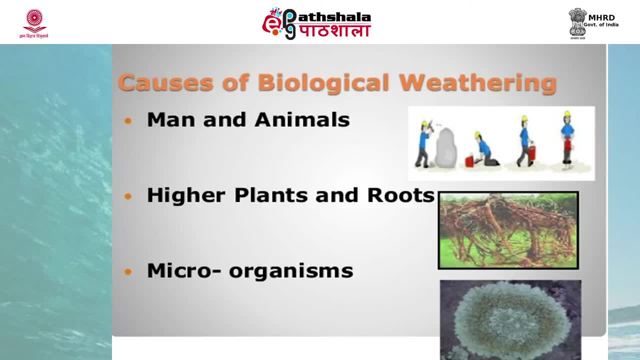 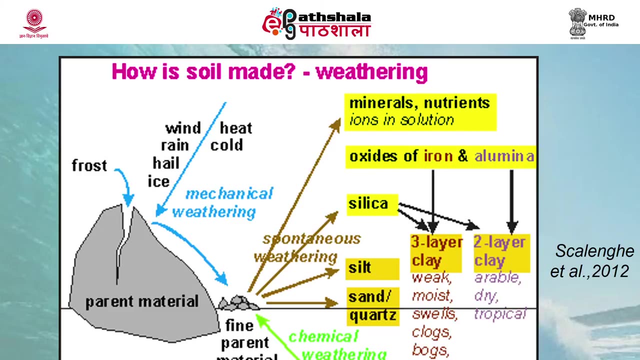 location in the soil profile. Simple chemical processes, like solutions, can be enhanced by the carbon dioxide produced by respiration. Carbon dioxide mixing with water forms carbonic acid. The complex chemical effects that occurs as a result of chelation. Chelation is a biological process where organisms produce organic substance known as chelates. 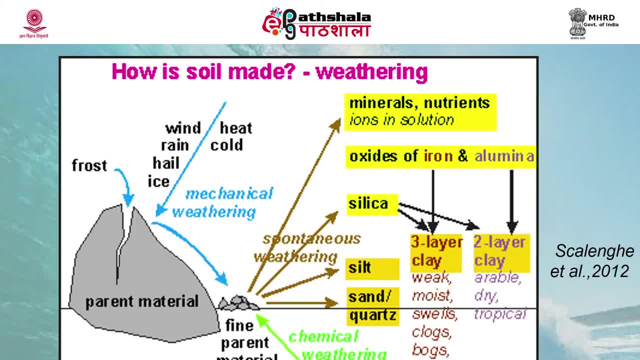 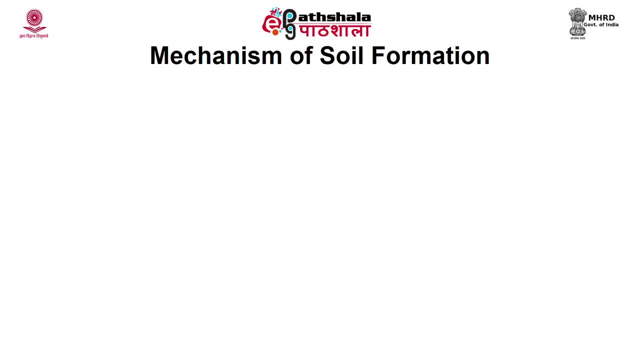 that have the ability to decompose minerals and rocks. by the removal of metallic catein Organisms can influence the moisture regime in soils and therefore enhance withering Shade from aerial leaves and stems. the presence of root masses and humus all acts to increase 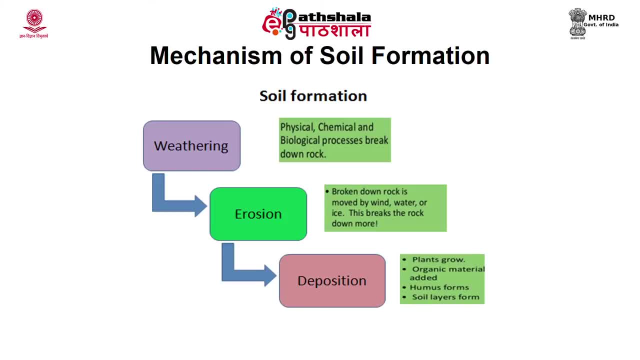 the availability of water in the soil profile. Water is a necessary component of soil structure. Water is a necessary component of soil structure. Water is a necessary component in several physical and chemical withering processes. Organisms can influence the pH of the soil solution. 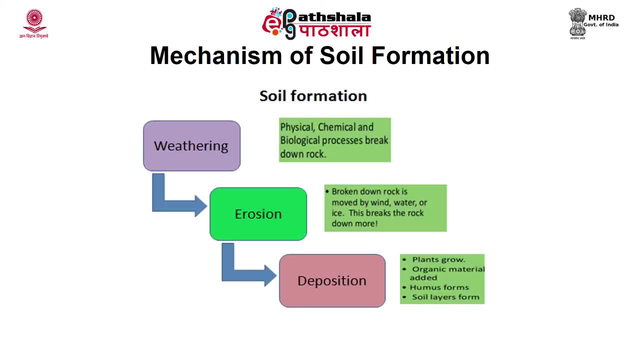 Respiration from plants, roots release carbon dioxide. If the carbon dioxide mixes with water, carbonic acid is formed, which lowers the soil pH. Catein exchange reactions by which plants absorb nutrients from the soil can also cause pH changes. The absorption rate of carbon dioxide can also be reduced. 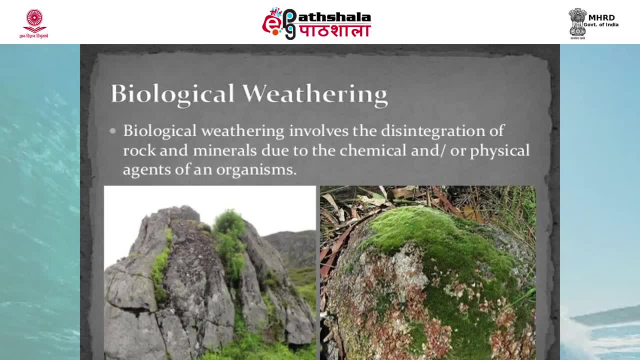 The absorption processes often involve the exchange of basic cateins for hydrogen ions. Generally, the higher the concentration of hydrogen ions, the more acidic a soil becomes. So these are also some of the important points that should be included in the biological withering process. 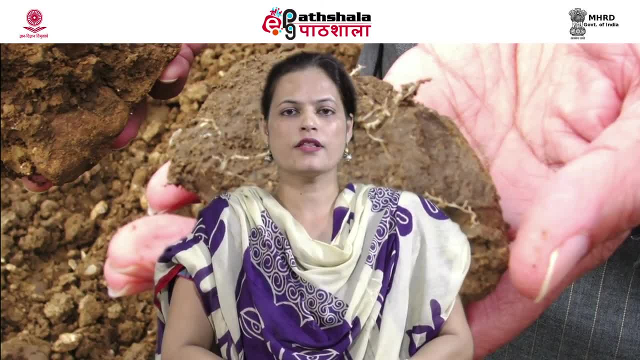 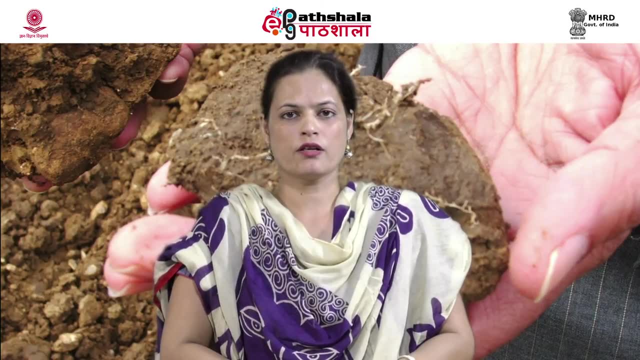 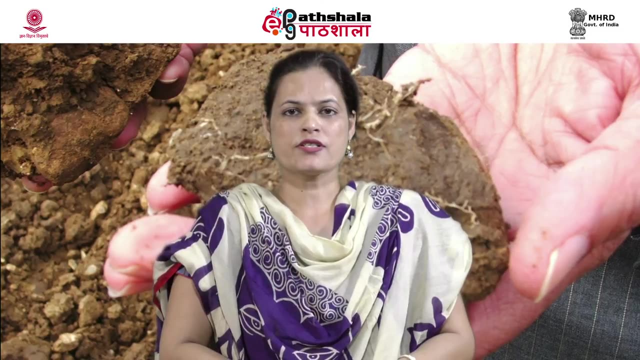 So in the conclusion, we can say that plants and animals, they also play an important role in the transformation of soil, Whereas, while transforming soil can also increase it or enrich itself by increasing its drainage property and nutrients within the soil. On the other hand, men are also responsible for the transformation of soil, either positively-